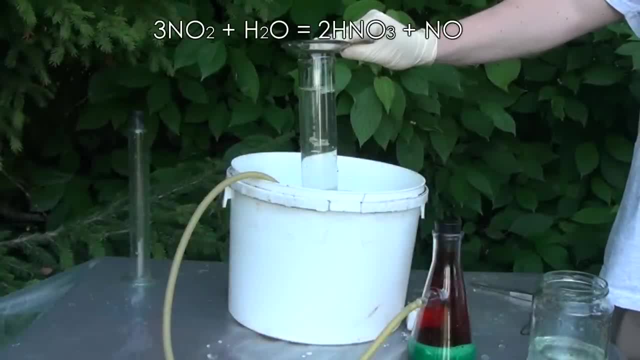 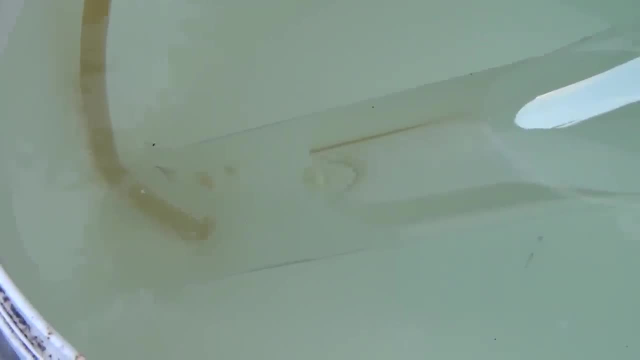 After this process, the nitrogen dioxide is released, Nitrogen monoxide which we pass through the water while it's reduced to nitrogen monoxide. We will fill such cylinders with nitric oxide, since they are usually being used to carry out the reaction. 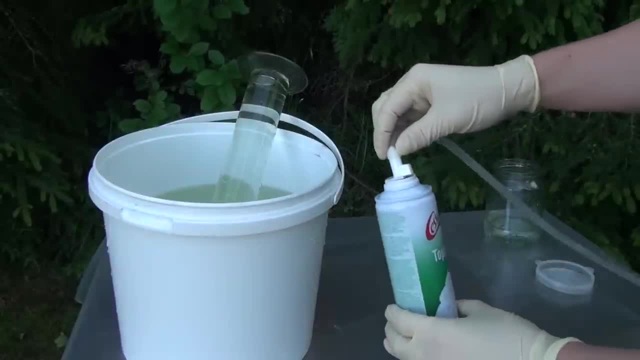 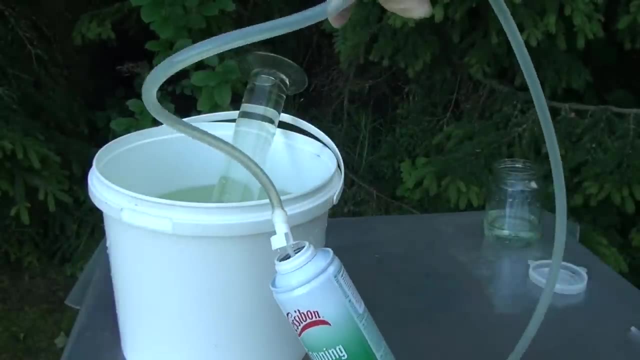 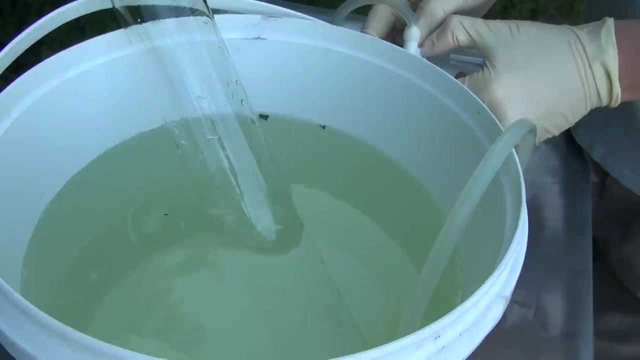 However, the reaction backing dock goes even better if you use nitrous oxide. An interesting fact that nitrous oxide is contained in bottles with whipped cream, which are sold in almost all stores. Nitrous oxide is eached off pretty easily and about 1.5 liters of nitrogen monoxide is released. 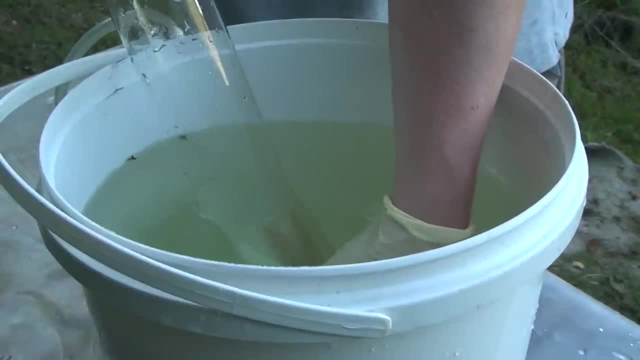 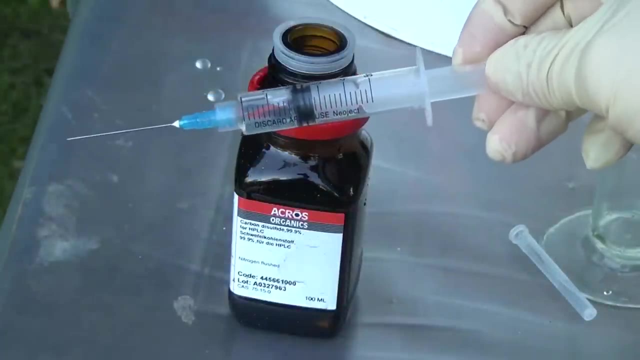 Nitrous oxide can be squeezed from one cylinder. After I filled all the cylinders with different gases, it's time to add the second component, carbon disulfate. Carbon disulfate is stored in these special banks, since it is very toxic. 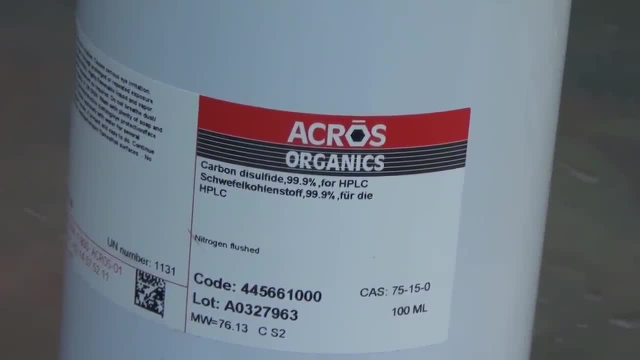 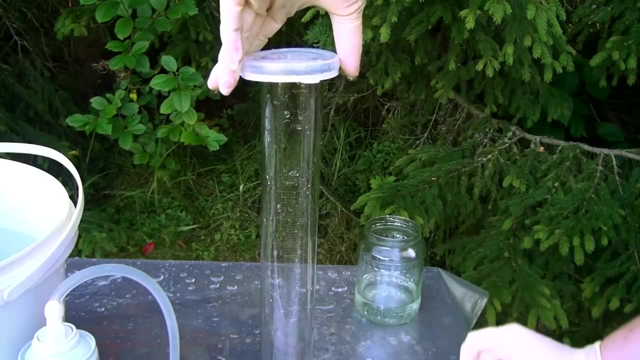 and work with it can only be done after acquiring the necessary special training. The ratio of carbon disulfate and nitrous oxide should be approximately 2 milliliters of carbon disulfate per 1 liter of gas After adding a small amount of carbon disulfate in the cylinder. 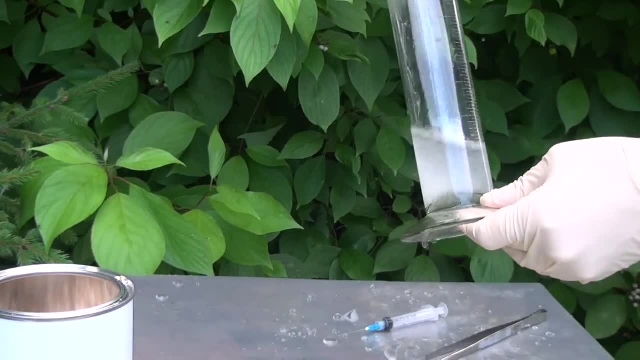 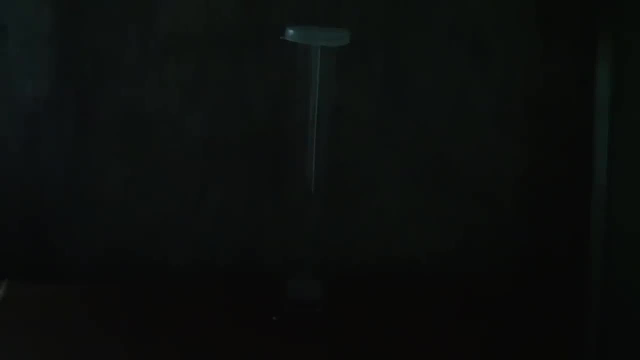 it should be mixed for the carbon disulfate to be evaporated, and mixed with nitric oxide. Well, now let's do the experiment. To start the reaction, I'm opening the cylinder and igniting the mixture of our gases. The reaction is very beautiful, during which a bright flash occurs, a so-called dog barking. 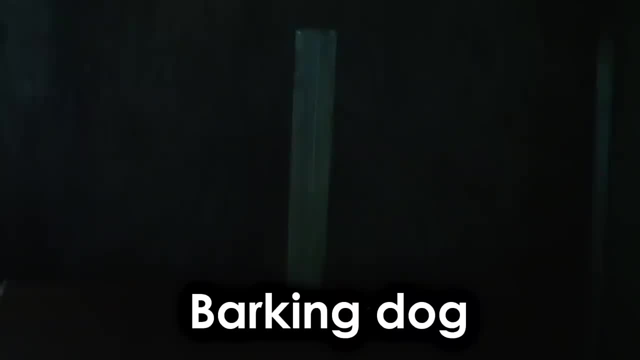 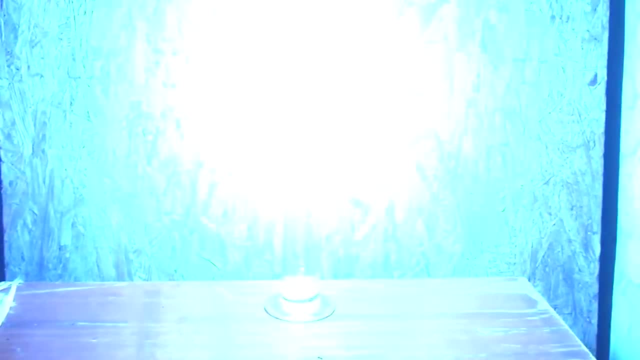 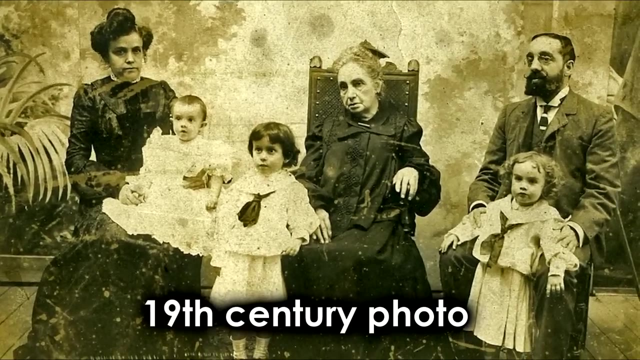 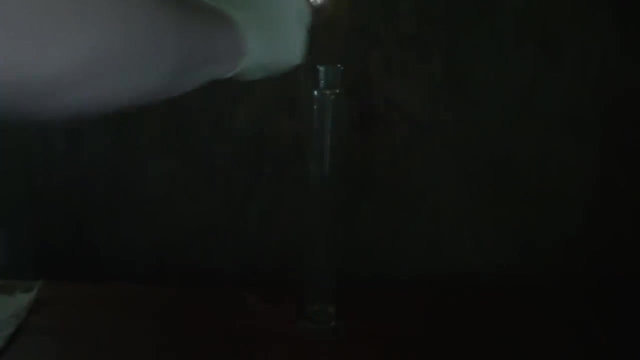 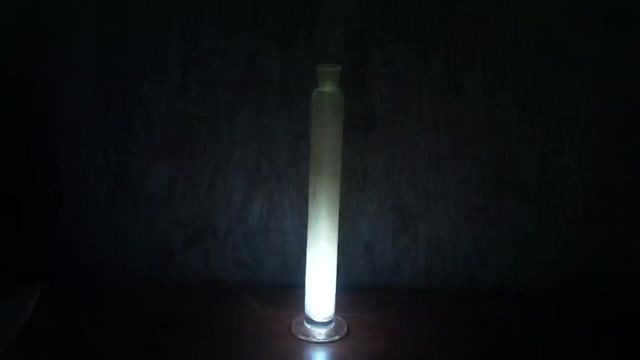 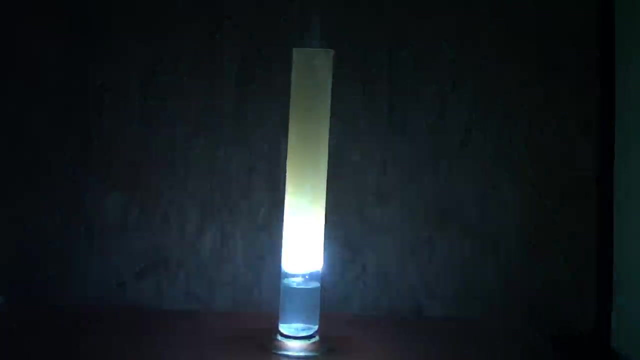 Therefore, this experiment is called a barking dog. By the way, I have an interesting fact for you. Before the invention of camera flashes, this reaction often has been used as an illuminator for photography. The reaction speed can vary based on how much carbon disulfate has been added.